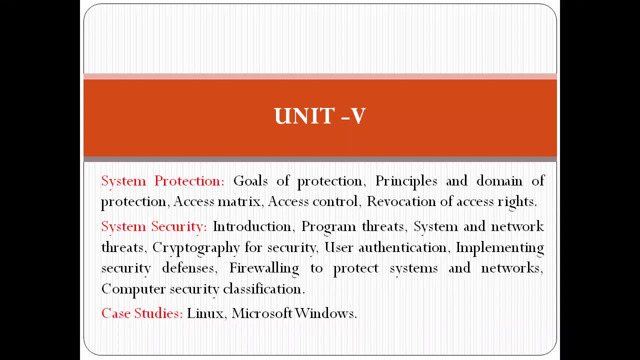 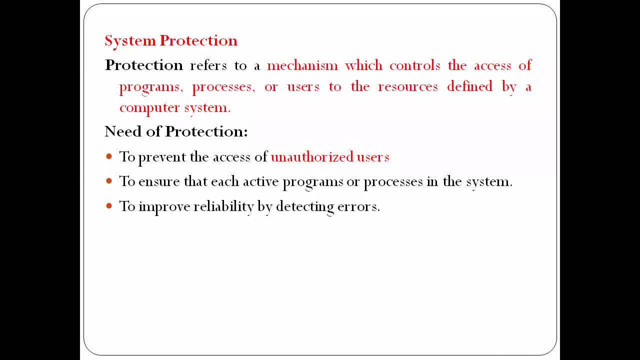 fifth unit, That is, system protection and system security. So, coming to our first chapter, that is, system protection. System protection: What is the meaning of protection? What is the meaning of protection? first, Simply here, protection is nothing but a mechanism which controls the access of programs, processes or any other. 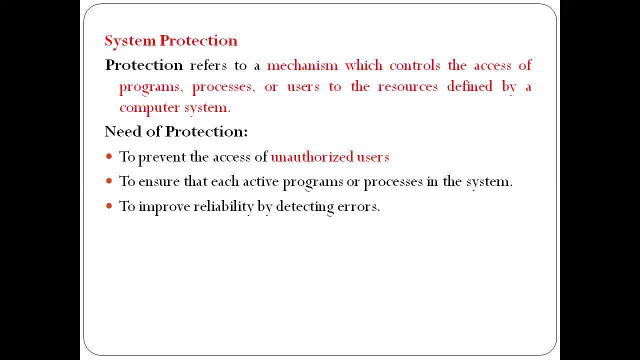 users to resources defined by the computer system. That is the meaning of protection. So simply we can call as: what is the meaning of protection here? Protection is nothing but control the access of programs or user to the resources defined by the computer system. This is nothing but protection. So what is the main need of protection If there is no? 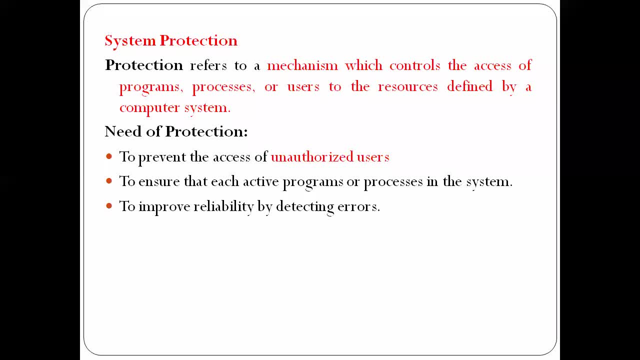 protection. what happened? If there is a protection, what happened? So there are different needs of protection. So first one is the main object of every system: protection is to prevent the unauthorized users, To prevent the access of unauthorized users. Who is unauthorized user? Authorized, unauthorized. 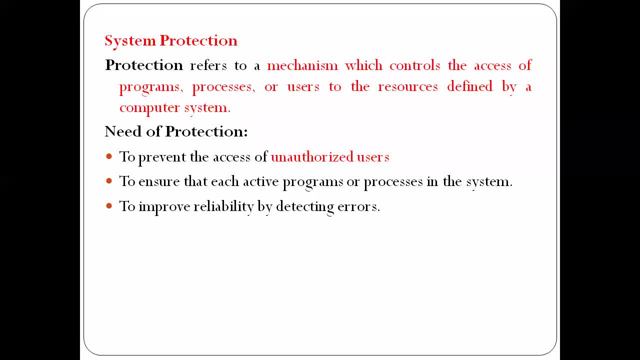 Who is authorized user, Who is unauthorized user. So authorized user is nothing, but, for example, this is my system, This is my system, So I am the owner of my system. I am the owner of my system. Right, This is my system, My system's information and also my system's resources. So what is? 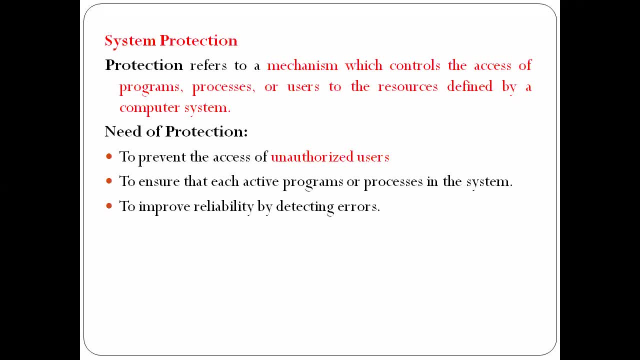 my system, For example, if you take, this is my laptop, So this is laptop of mine, So I am the owner. So not only laptop. Laptop is nothing but a hardware, Not only laptop, For example, laptop. My laptop consists of some valuable information. My laptop consists of: 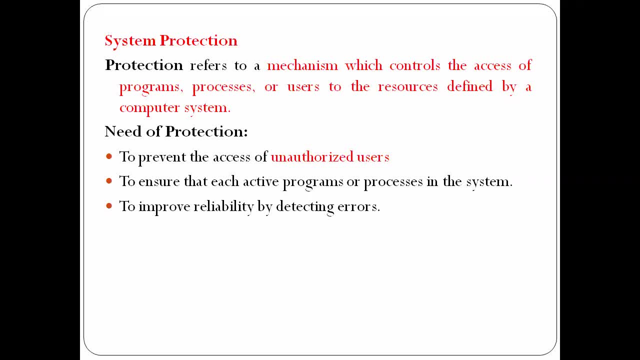 some valuable information. So this information belongs to me. This information belongs to me. My valuable information is: Who is that information? That valuable information belongs to me. So I am the owner of my system. System is nothing but hardware, And also I am the 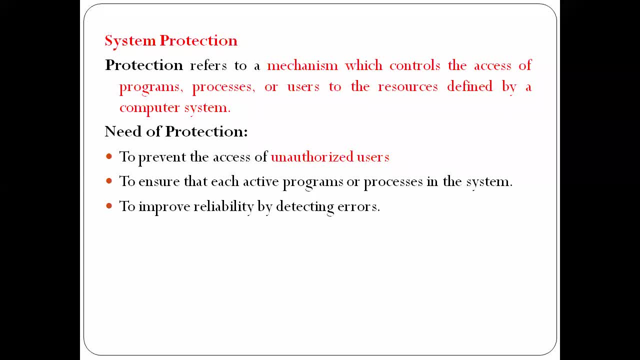 owner of my system's information, System's valuable information. Okay, So if I want to access my system and also my system's information, So I am the author of the person, So I am the author of the person. Who is the author of the person? Author of the person is nothing but Author of the person. 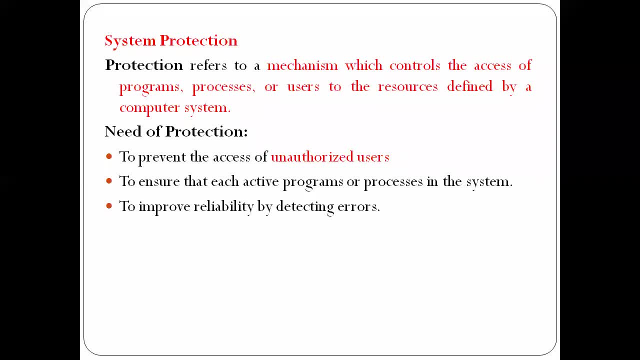 is nothing but owner of that particular system or system's information, Who is unauthorized person. So this is my system without my permission. Without my permission, some X person want to access my system and also my system's information without my permission. That person is called. 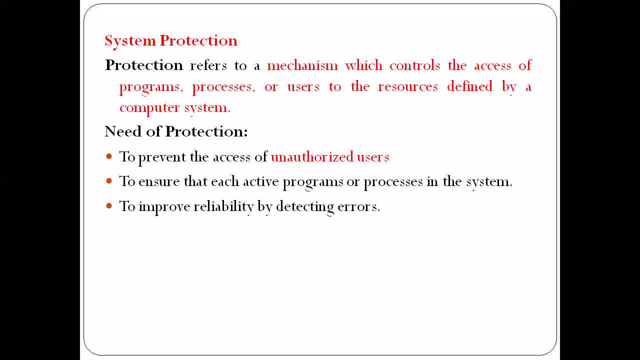 as unauthorized user. So simply we can define who is unauthorized user. Unauthorized person is nothing but accessing- accessing someone's information, Someone's system and also system's information without owner's permission. That person is called as unauthorized user. So simply we can say: 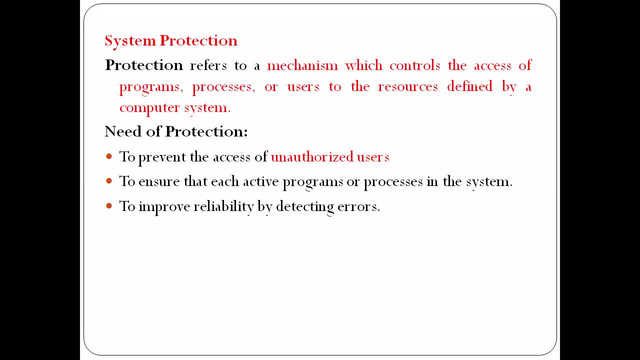 unauthorized person is nothing but hacker. Okay, Here unauthorized person is called as hackers. Okay, So what can do my valuable information Unauthorized person? what can do? So unauthorized person may do some unauthorized activity with my valuable information. So we must select. we 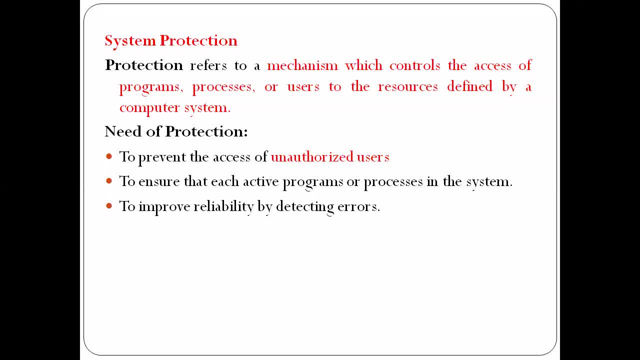 must protect. we must protect my system, and also system's information, from unauthorized activities or unauthorized user. Okay, Okay, Okay, Okay. So our first need is to prevent the access of unauthorized user. That is our first goal, our first need of our protection. Next one is to ensure that each active program or process 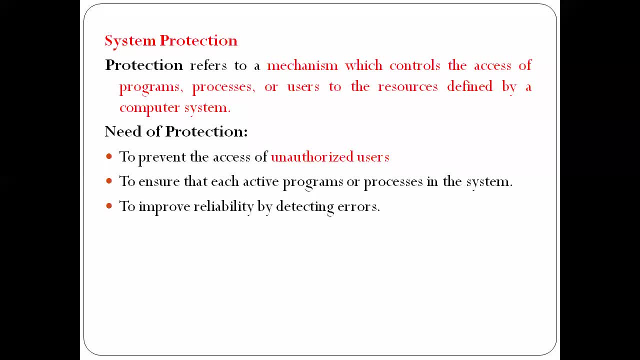 in the system. So our second need, what is that? So to ensure, to ensure each active process, which is active process, which is active program or which is inactive process. So those all are ensured with the help of our system protection. Okay, 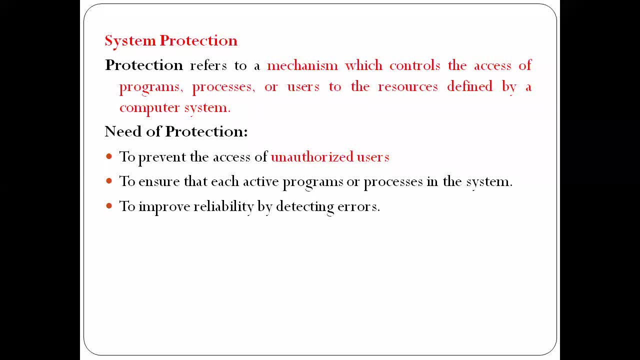 Okay, our system protection. okay, now coming to our third one, that is, to improve reliability by detecting errors. ah yes, this is another best need, and okay, so another best need is another best need of system protection is to improve reliability by detecting errors. what is the meaning of reliability? 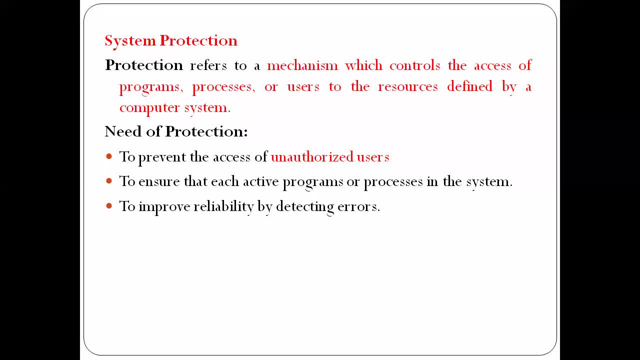 what is the meaning of reliability? reliability is nothing but a guarantee of service, guarantee of services. so simply here, reliability is nothing, but if your system is failed, then other system will provide the same services of the train system, example, atm systems. okay now, for example, if you withdraw, if you want to withdraw thousand rupees from this atm, but unfortunately this 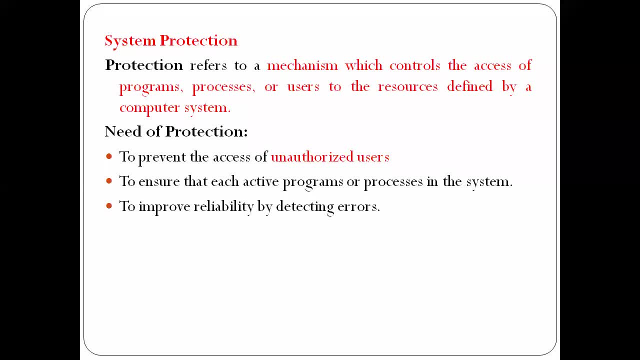 agent is failed. what happened so you? you go other atm and then, and then with the same thousand amount, say thousand amount, how? for example, if you want to perform this atm but unfortunately this item is performed, so other atm through other atm, or you can get same services of this failed system. 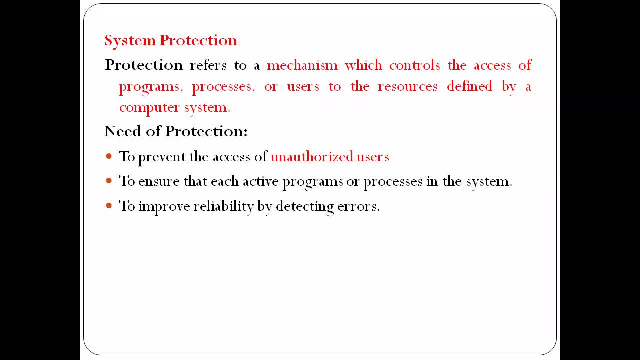 so this is nothing, but this is the best example of reliability. so here, another need of a system protection is to improve reliability by detecting errors. okay, so these all are some needs of production. okay, now, in this there are two, uh, there are two best needs, and the first one is prevent unauthorized users from unauthorized activities, and next one is: 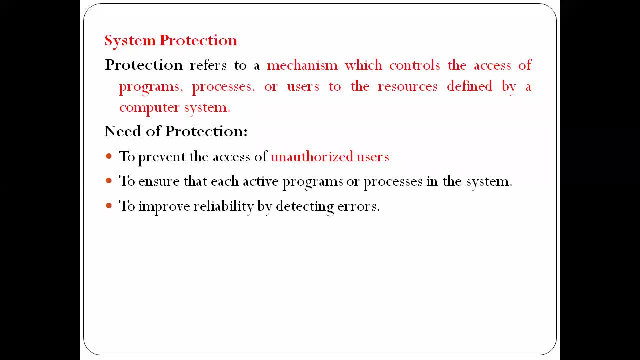 reliability by detecting errors. these two are needs of protection. okay. so, simply, what is the meaning of protection? system protection? system protection is nothing but the mechanism- system production is nothing but mechanism which controls the unauthorized users from unauthorized activities. okay, to control the access of the system. which controls the access of the system. okay. so the other two needs are programs or processes. 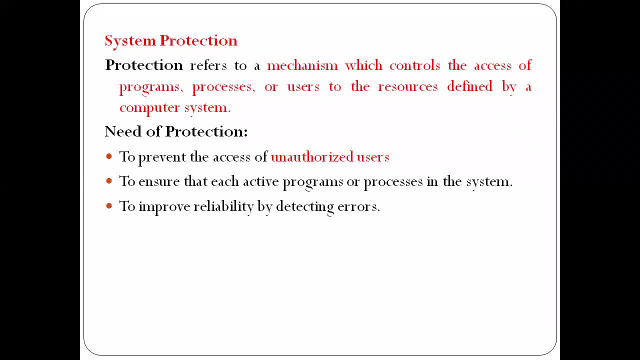 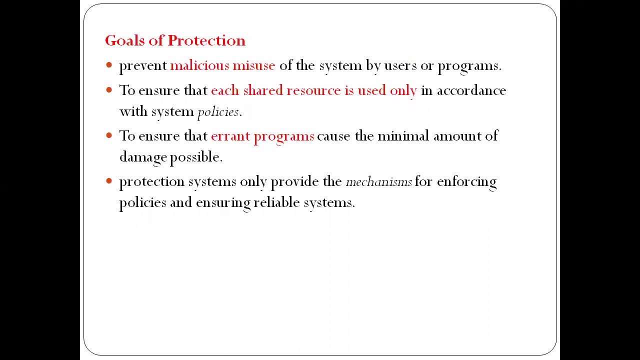 or something users to resources defined by the computer system. this is nothing but system protection. okay, and the main needs are: first one is prevent the other activities and next one is improve the reliability to detecting errors. okay, these all are some needs to protection. next one is goals of protection. goals of protection, you can simply these three are. these three needs are nothing but system protection. 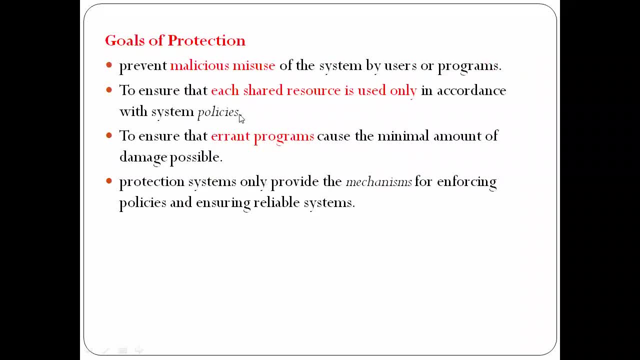 goals. these three are nothing but goals now, especially we defending some goals of protection. first goal is prevent misleases, misuse of system by user or program. so simply, this is. another is the activity okay? so simply yes. what is the meaning of this? so our first goal is: protected. 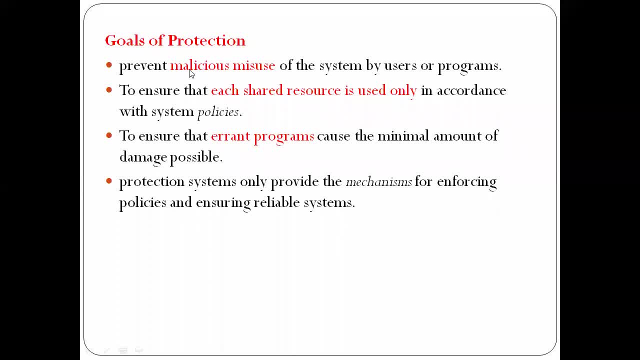 misuse of the system by user or program. so, simply, what is the meaning of malicious? what is the meaning of malicious misuse? what is the meaning of malicious misuse? simply, this is an average activity, okay, so we define here. so another name of another user is nothing, but here malicious misuse. okay, malicious is nothing. 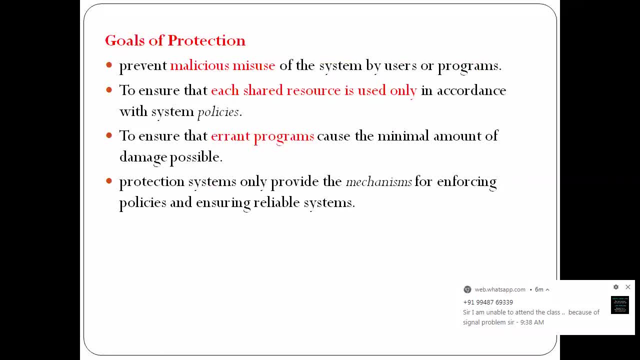 but he, he can, unknown person, he can- perform some an average activity without permission of the owner. so that is nothing but malicious misuse. okay, so simply. malicious misuse of the system by user or program. that is our first work. okay, so simply. our first goal is to prevent the unadvanced activity. next one is to ensure that each shared resource is 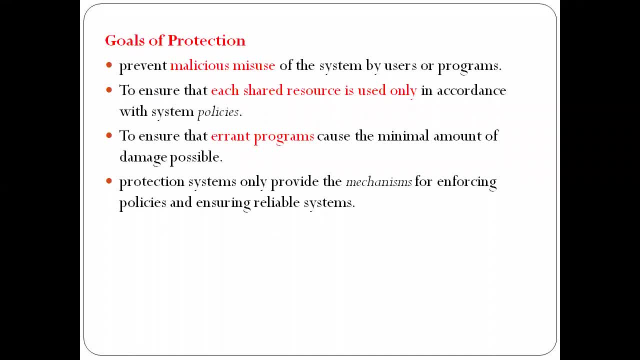 used only in accordance with the system policies. okay, just what is the movies, for example? this is my network system. my network system consists of: uh, network system system, one printer, one scanner, internet connection, these are all things. so here our goal is what is? to ensure each shared resource? 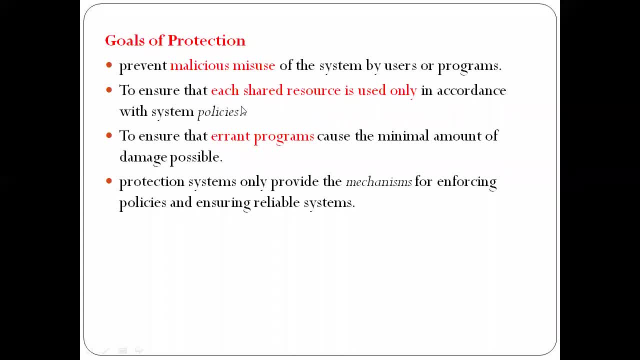 is used only in accordance of the system policies. okay, system policy, center media injury. so, in a total of connective and devices, my editing works are done to ensure that each shared resource is used only in accordance with system policies, not beyond that. okay, now coming to our next goal, that is, to ensure that 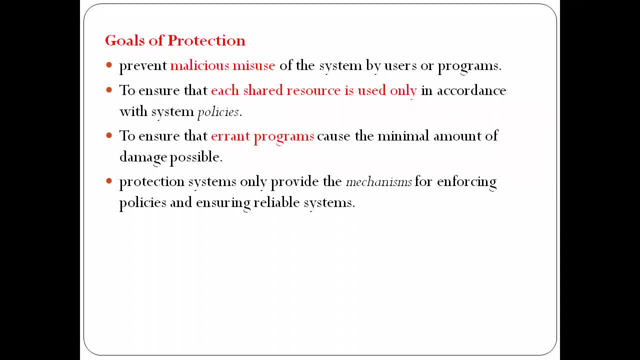 error programs. what is the meaning of event iran is nothing but temporary, cannot prevent is nothing but temporarily. so this event program can can damage e programs in the current programs, some temporary programs and the e programs and every worker systems ecosystem. actually these programs are not harmful to the system. 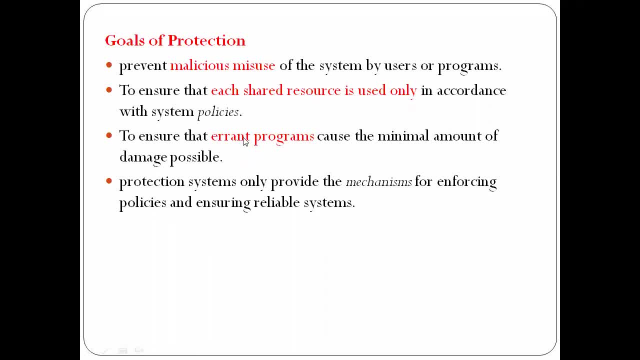 if, okay, if user unable he attends programs, he can control it. it may damage our system. okay, it may damage our system. so these programs move one system to another system continuously, okay, so if user uh not control this particular event program, what happened? this program may damage our system. so simply, our here. our next goal is to ensure that internet program. 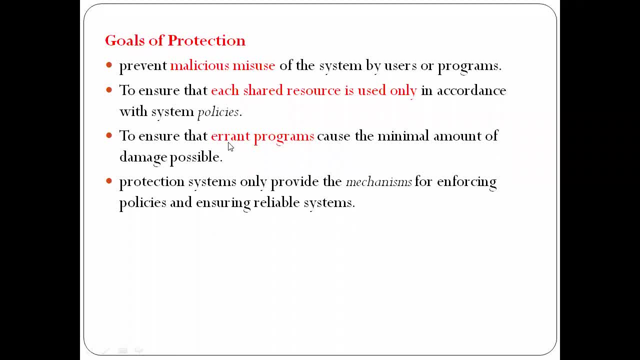 does the minimum amount of damage possible. okay, so simply control the event program. that is our next goal. next one is protection system only provide the mechanism for enforcing policies and ensuring a reliable system. so simply reliable system. okay, simply reliable system. so our goal is: our goal is improve the reliability of the systems. so these all are the protocols of protection. so 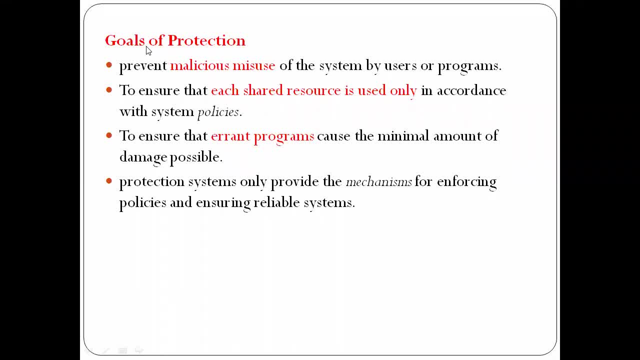 i am simply concluding these goals once again. so goals of protection: our first goal is prevent the unauthorized activities, nothing but malicious misuse. and next one is to protect the each shared resources- okay, each shared resources from from accordance with system policies. next one is: okay, to control iran programs, otherwise these events programs will damage our system. next one is: 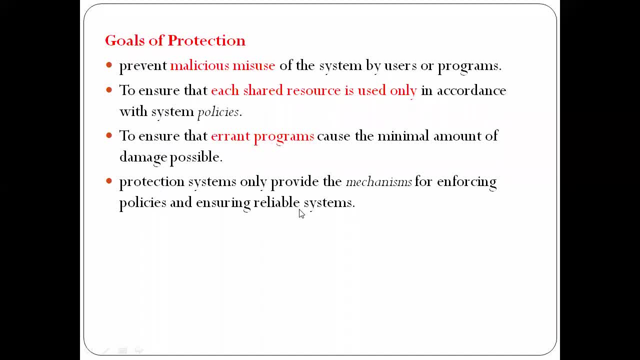 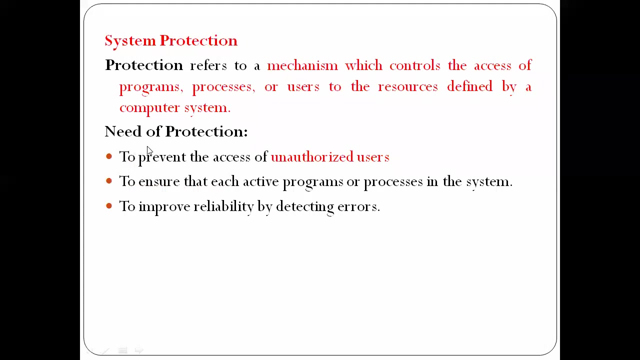 improve the, improve the reliable service, improve the reliability of the system. so these all are the availability of settings. okay, so these all are goals of protection. okay, so equals. in charleston 7 refugee challenge, anything is different. define protection. explained goals of protection, explain about goals of protection. so you must explain these all things, okay. so first one is protection. 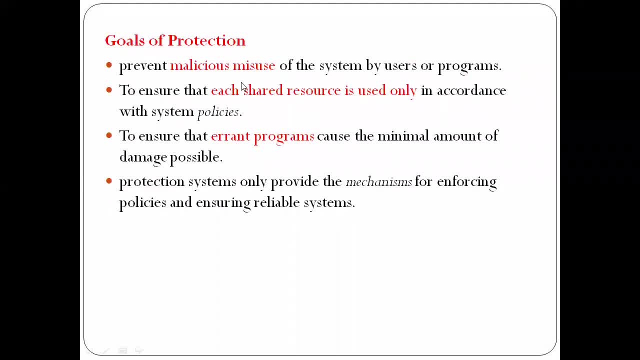 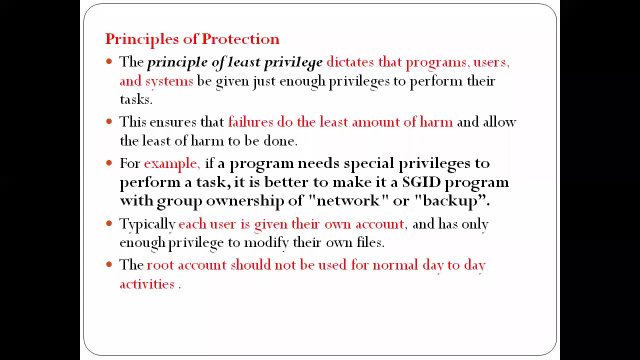 definition. next one is need of protection. next one is supposed to protect you seven months. okay, now coming to our next one, that is, principles of protection. principles of protection, yes. what is the meaning of different principles to protect? okay, there are different principles. these are principles are used to. 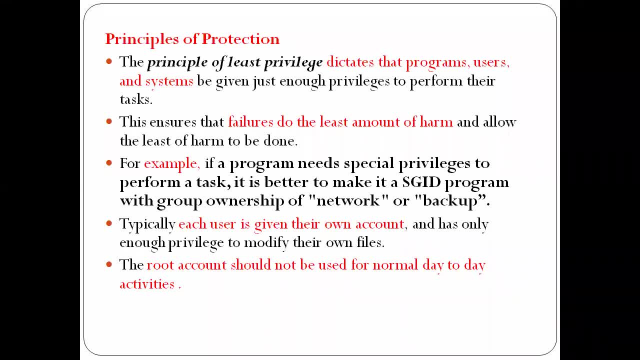 protect the our system. okay, first one is first, one is okay. first of all, principle of least privilege. yes, what is the meaning of privileges? okay, what is the meaning of privilege? privilege is nothing but giving these some permissions to do, to do some tasks. privilege is nothing but here. what is the meaning of privilege? here, privilege is nothing but. 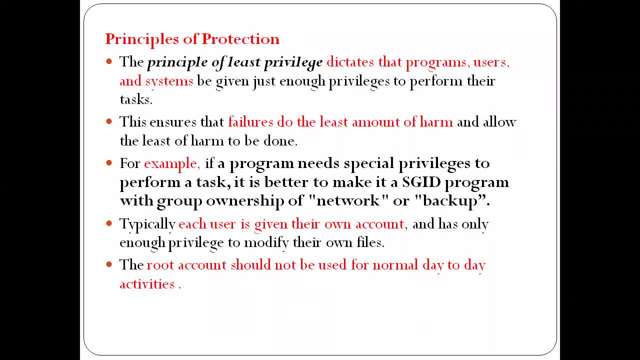 giving the access or giving the permissions to perform some tasks. that is the meaning of privilege. okay, so, principles of protection, our first one is principle of least privilege. their privilege is nothing but giving some permissions to perform some tasks. okay, so here, what is happened here? so in a network system for 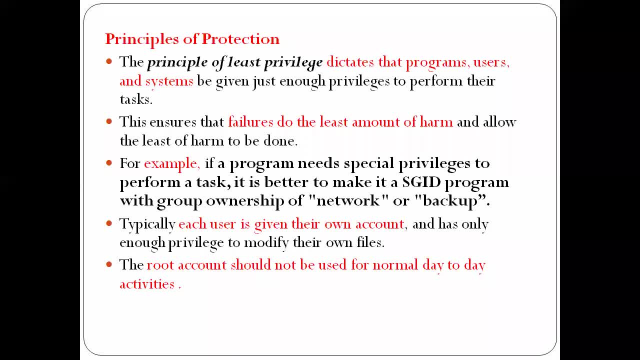 example, if you take a software company or something, any other company, so here each and every employee, each and every employee can have some privileges to do some tasks. okay, they can only perform. they can only perform the task only, not beyond that. why because? why? because each software employee or each user consists of some limited privileges. okay, so privileges is. 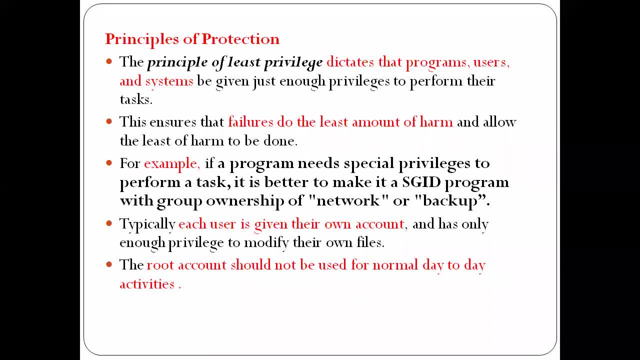 nothing but previous, define those person perform some task only so all persons consist of same privileges. now, these are all employees. all users can start saying to this: you know, some employees can just have some privileges. some employees consist of some privileges. okay, so some members consist of some uh high privileges. that means, for example, if you take our college, our college. 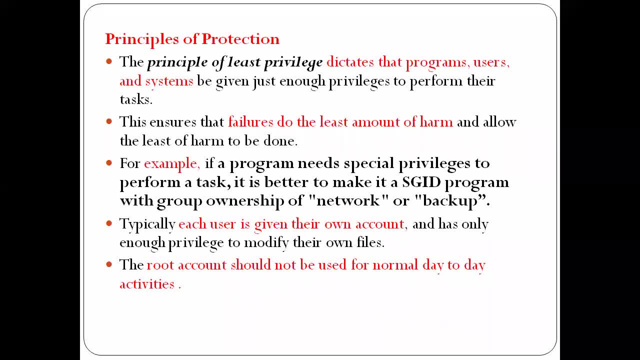 uh, principal consists of some privileges. okay, hod is consisting of some privileges. normal advice, nothing but staff consists of some privileges. programmers can step some privileges. okay, non teaching can have some privileges. they can perform only that particular task, not beyond that. so simply, privilege is defined. privilege define what? 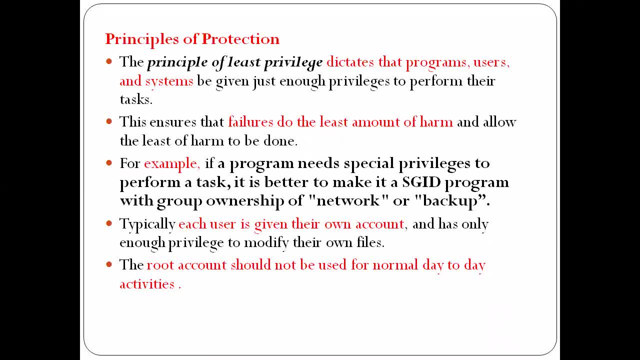 define what some access permission. privilege depends on access permissions they can perform only with their task. only now, what is the main objective of privilege? to secure nothing but to protect the system. so privilege one usually, if we will not actually generally, or whether, for example, teaching e-tasks. 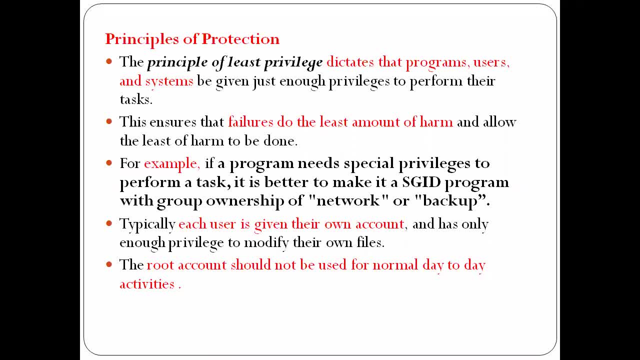 you didn't define even privilege system. so to protect the system, privileges are must. okay, so these privileges detect that programs, users and assistants- okay. what is the main object of discovery is these previous are used to detect that programs, users and the system. okay, so system need protection users as well as system. 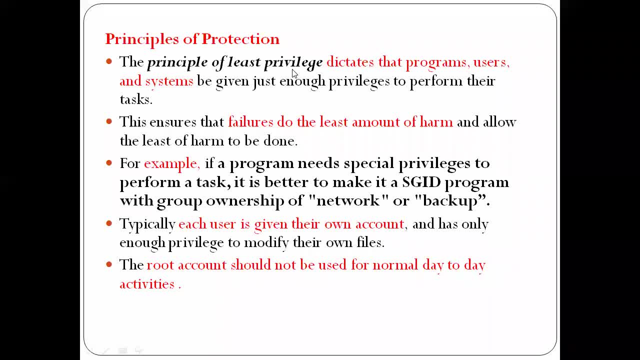 software. okay, next one is next question. next one is to ensure that failure to the least amount amount of harm. what is the meaning of this? for example, if the failure is happened, if the failure is happened, the failure must be least amount. the failure must be least amount. okay, for example, any precautions? 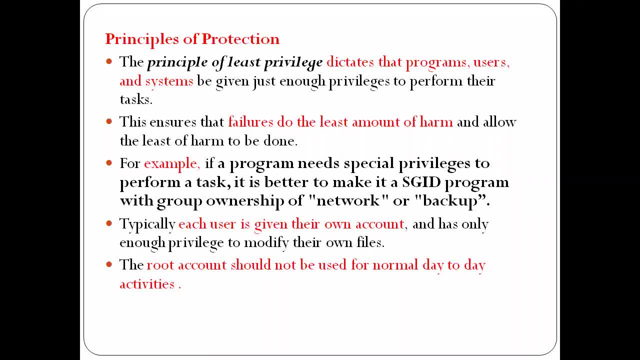 any previous, any protections. this is not either failure of any previous. we can see here in the space from the scenario we can see here in the view. we can see the last one. we can see here in the view. we can see. we can see the other end of the picture in the library. 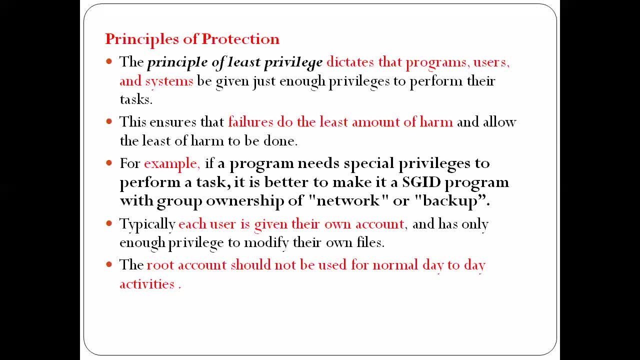 so if the failure happens, then the system will not be there. the system will not be there during the time period. so we should be careful. in the first case, we are following the same rules, okay, so we are following the same rules, okay. so you guys can understand what it means. 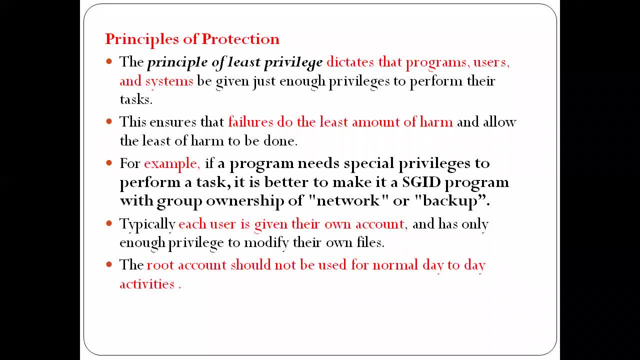 okay, okay, After that, there shouldn't be too much damage to us. So if there is an accident, the damage shouldn't be too much, Same as if a failure has happened in the organization or in the system. failure will do the least amount of harm. 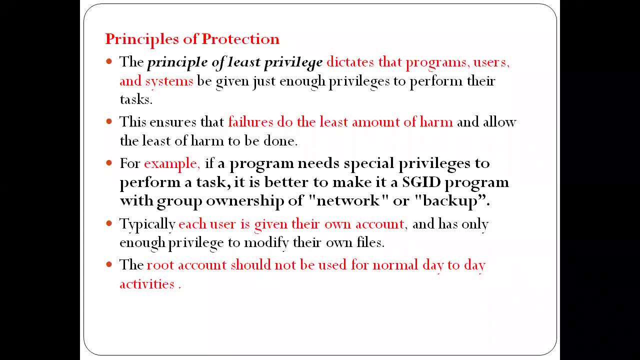 That is the principle. That is the second principle. Many a times we say in COVID, get vaccinated, get vaccinated, get vaccinated. But no one can say that getting vaccinated will cure COVID. Even if COVID comes, it will go to death. 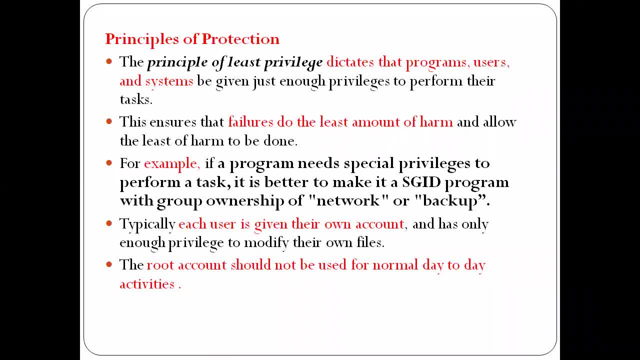 What is the use of getting vaccinated? COVID may come, but if it comes it will not go to death. It will go to death. It will be just a small symptom, That is nothing. but that is the same example. Feel you to the least. 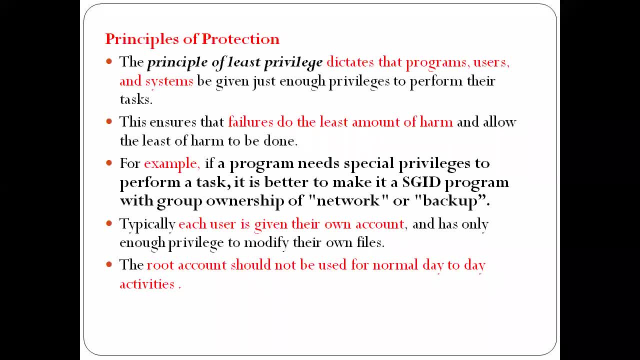 That is the principle. Here there is a simple example How an organization consists of principles of protection. For example, if a program needs special privilege to perform a task, it is better to make it as SGID. SGID is nothing but. 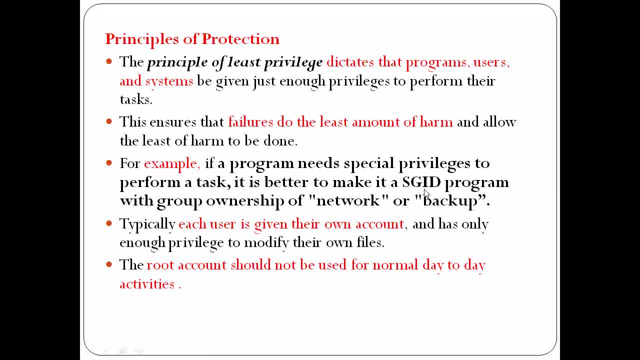 for example, that is login ID. For example, SGID is the login ID. For example, if a program needs special privilege, that program needs two special privileges. So there is a company. In that company there is a small program. 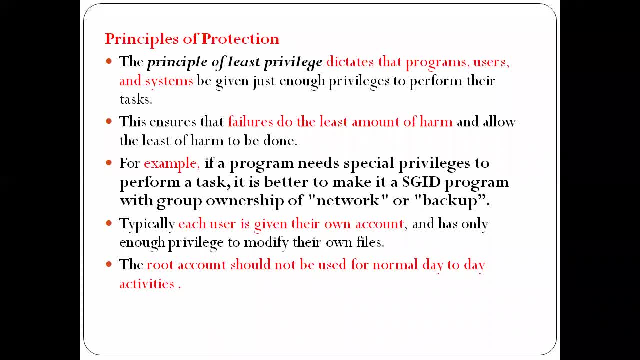 That program is a special program. That is a very important, very sensitive program. So to access that program everyone is not allowed, Only a few people are allowed. For example, we gave permission to a few people, Then we gave an ID. 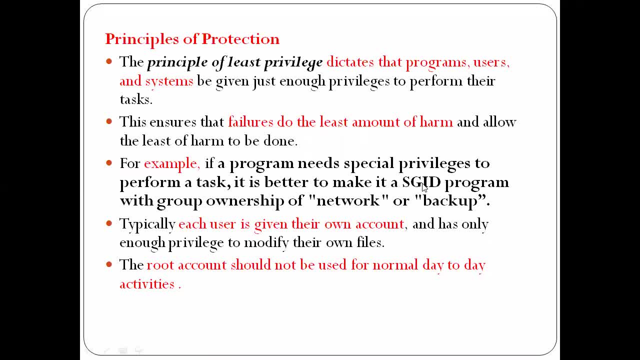 That ID is called SGID. SGID is nothing but login ID. So with this SGID the users who have this particular user ID that is SGID, the user can access this user ID and perform some task or can unperform some task. 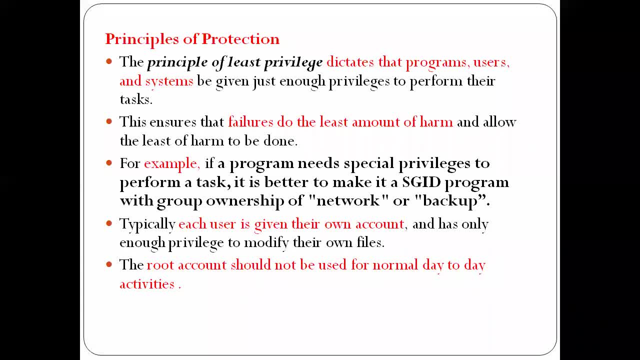 and then log out. So what are these people doing? So whoever accesses that program at the same time, if they access it, they are limited persons, only If they access it carefully, if there is any modification or something. if there is any modification. 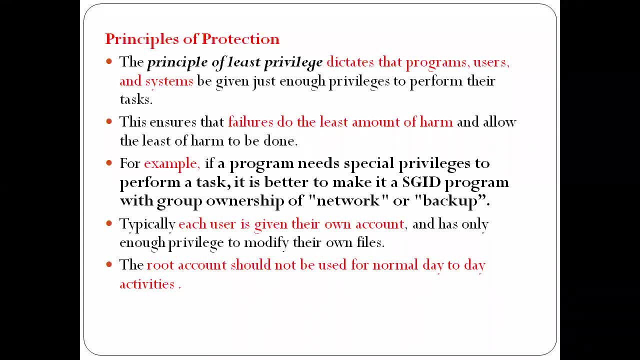 it will be back up again, So because of this, you can use this valuable program without misusing it. The simple example is: for example, we have a password for Wi-Fi. We have a password for Wi-Fi, For example. 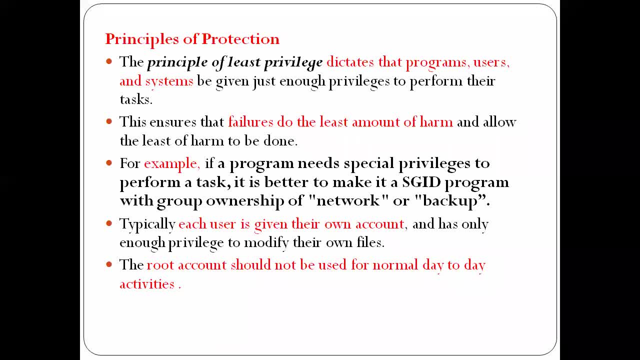 what is the use of a password for Wi-Fi? What is the use of a password if someone has an open account? Tell me. If it is open, who will use it? They will corrupt the entire network. That is because of the password. 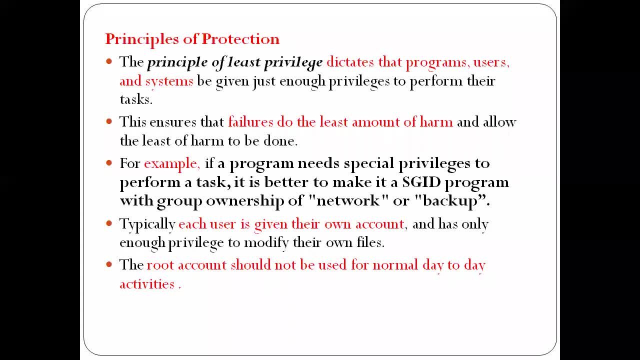 Only, for example, if there is a Wi-Fi in our college, that Wi-Fi should have a password. What does that mean? So whoever works in that college, all the employees of that college know that password and they can access it easily. 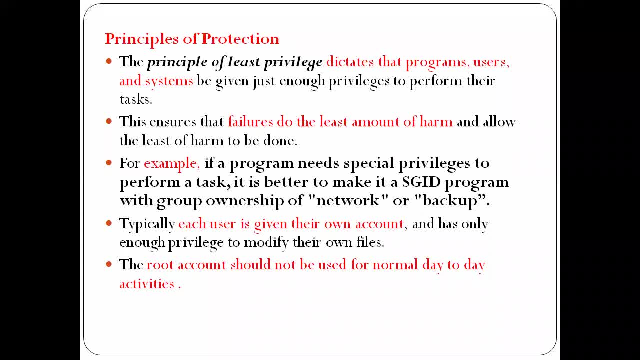 For example, a new person came. He ended the Wi-Fi, So the Wi-Fi will be detected, But he is not using it. He is an unauthorized person. He is not our college person. If he is our college person, he will be guaranteed. 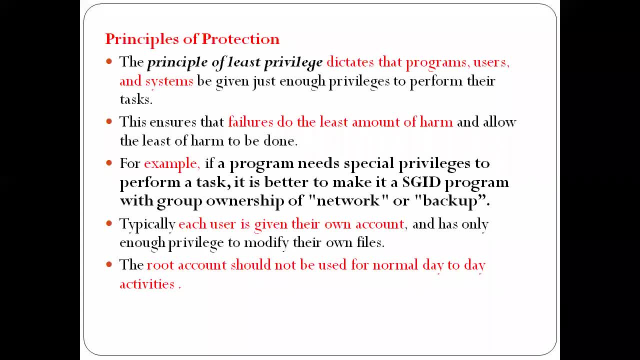 to be given a user ID, But he is not our college person, So he did not give a user ID. Or he did not give a user ID password, So he cannot access it. So simply, what is the meaning of this? 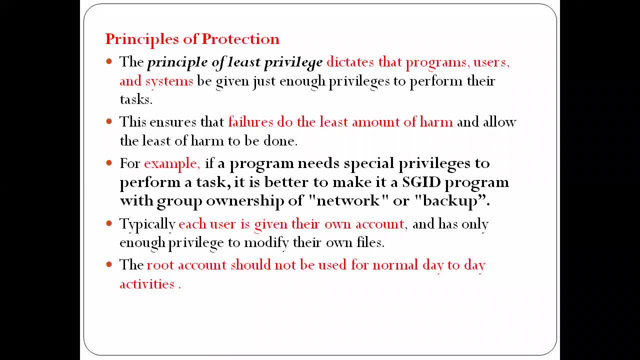 Here in any organization to access some valuable information. what happened To access valuable information? all users are not permitted. Only some specific authorized persons are allowed to access that particular valuable information using some SGID. Here, SGID is nothing but. 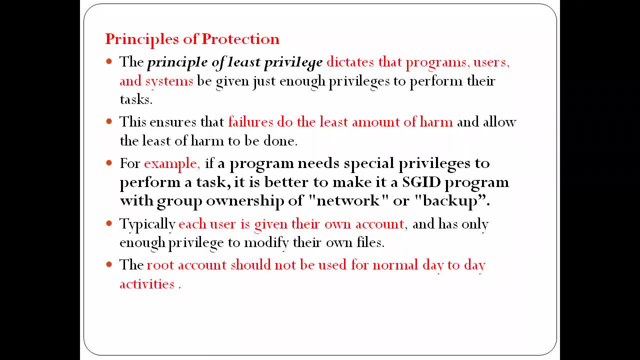 Special Guest Identification SGID. So simply here using here ID SGID, you can access that particular valuable information using some SGID. Here SGID is nothing but Special Guest Identification SGID, So simply. 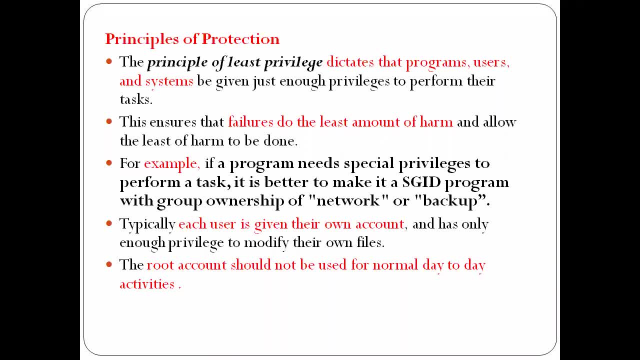 SGID is nothing but Login ID. Using this SGID, those specific, those limited persons can access that particular valuable information and also simply log out after the completion of that particular usage. Okay, So if any updates are performed, those updates are. 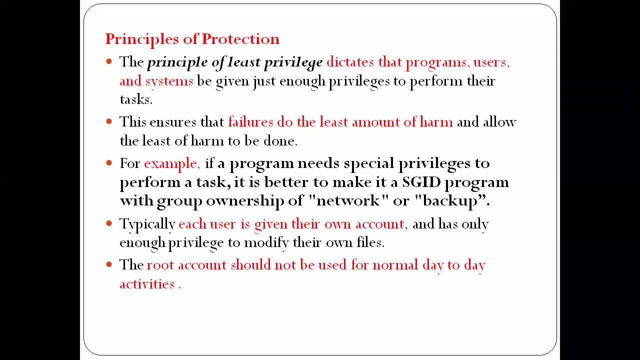 recorded as backup. Okay, So in this way we can protect. In this way we can protect. Okay, So kind of wurden can look good like this: nothing, mostly like someone which was totally persistent. okay, that only so. the the 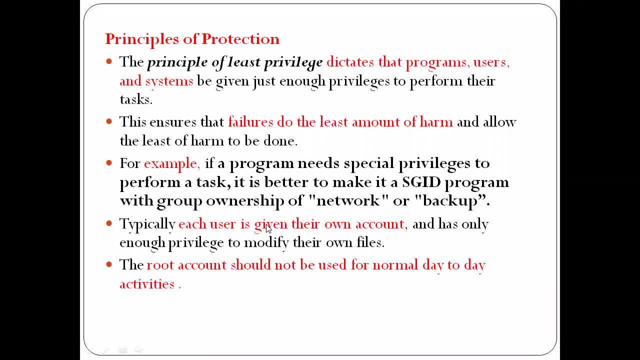 questions first, through course can be satisfied after maximum situation. if there have you any concern this days, okay, normal day to day activities. what is the meaning of these? so simply here, esg ids are only for specific persons. for example, if uh organization consists of 100 employees in 100 employees. 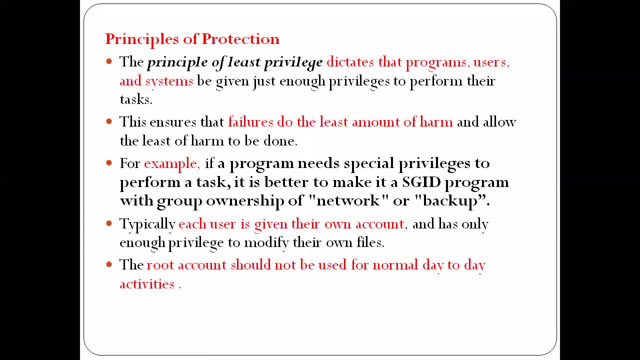 there is a one employee that is the manager. i think he is the boss. boss consists of a root account. boss consists of a root account. what, what he can do? he can do only specific tasks. he can do only specific tasks. that is his job, boss, okay, boss is the boss, is the upper person. 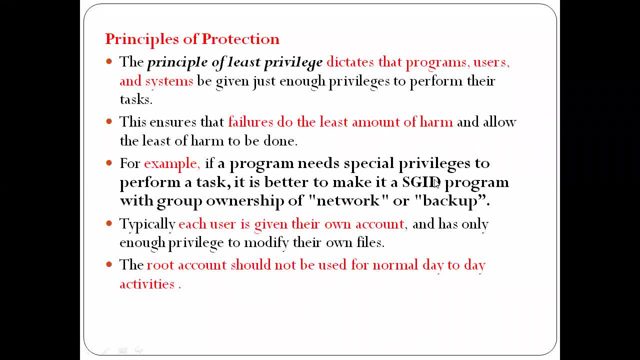 but not normal day to day entities. okay, for example, some of the wall and just control wall, one of our voices, so simply, what happened here in every organization? okay, in every organization to protect that valuable information, there are some ideas are given. okay, some person, some sgid, some personalities, one person can stand, some group? 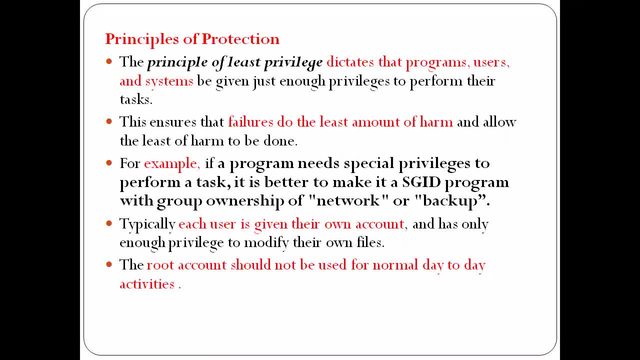 account, broken account. he can control all. he can control hours. so these all are why these all are. these all are used to protect the system, system, system. i mean any organization should not be able to control all these all are. these all are used to protect the system system. 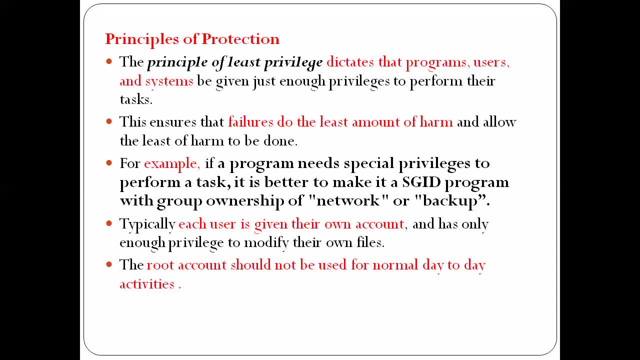 not only system, systems, information, also from another activity. so, simply, this is nothing but used to serve production. okay, simply, i am regarding this topic again. okay, what is the meaning of this? will see, there are two histories are defined. what are those first one is privilege. what is the meaning of privilege? privilege is nothing but privilege is nothing but allow the 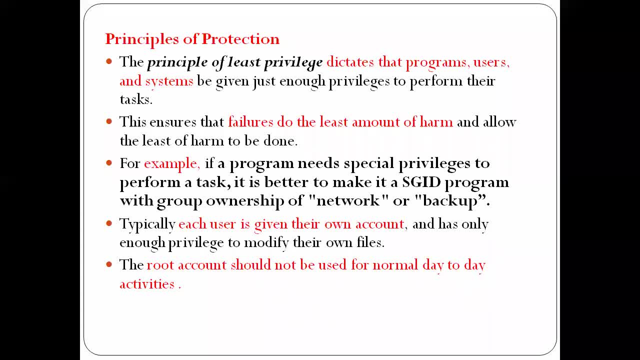 privilege is nothing but allow the, allow the particular person to do something. that is the meaning of privilege. okay, what is the main use of this privilege? the main use of this privilege is nothing but to control the axis. to control the axis, okay, and prevent the unauthorized activities. 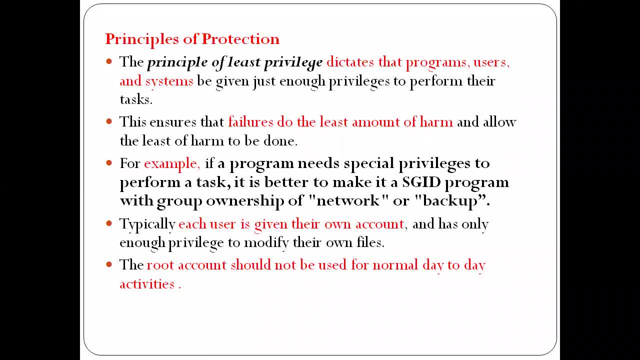 okay. next one is if these all precautions are taken, but some failures happen. so how these fields? there is a simple example is given. okay, in every organization or something in the organization there is some independent, some sgids. so sgs are nothing but, uh, simple ideas. using these ideas. 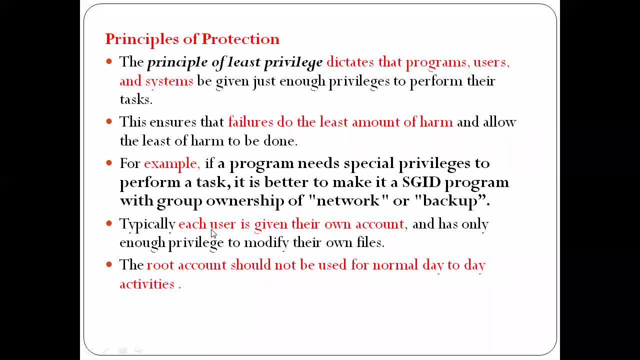 user can perform their own task only. yeah, there is another. some normal ideas are there? so using the can perform with their own accounts. okay, there is a one group account. he is the administrator, okay, but he can do all tasks but he cannot, uh, use the for normal day-to-day activities. so this is about 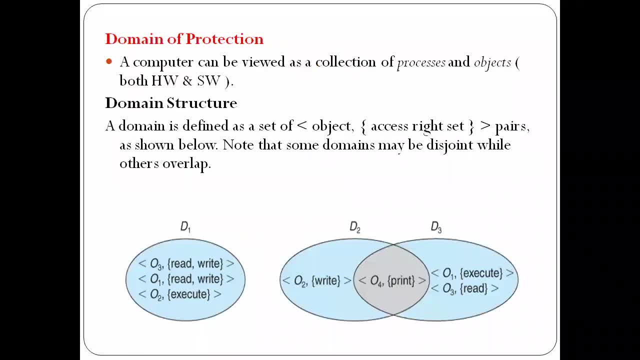 our principle self-function- okay. next one is domain protection- okay. next one is going to protection. what is the meaning of domain protection? okay. now what is the normal domain protection before that protection? what is the meaning of domain? what is the meaning of domain? domain is nothing but category. domain is nothing but particular category, particular group- okay. 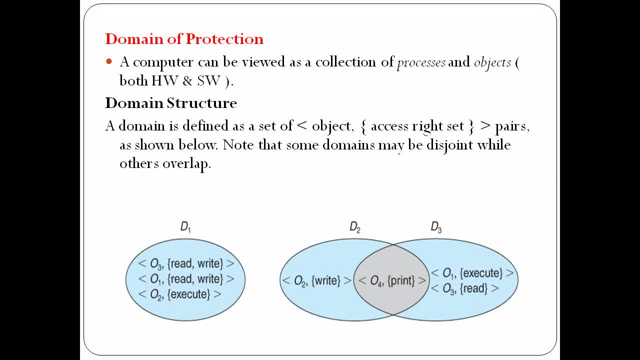 particular group. so simply, domain protection. what is the meaning of domain of production? so simply here. every computer consists of collection of process and objects. every computer can be viewed as collection of process and objects. what are those here? process is nothing but process is nothing but software. objects are nothing but hardware. okay, 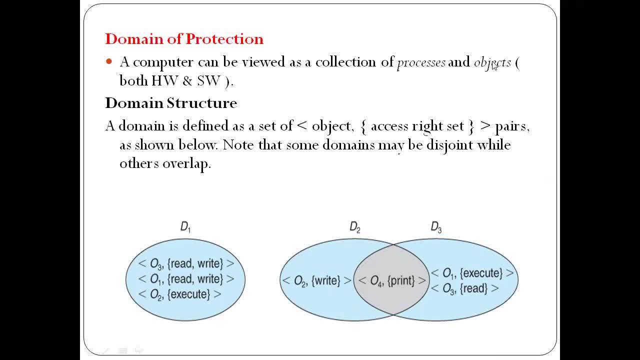 objects are nothing but keyboard, monitor, mouse, processor, cpu, these are things. process is nothing but software. it may be application software, it may be a software. okay, so process is nothing but software. objects are nothing but hardware. so simply we can say: computer consists of a collection of hardware and software. simply we can say: computer consists of collection of hardware and software. 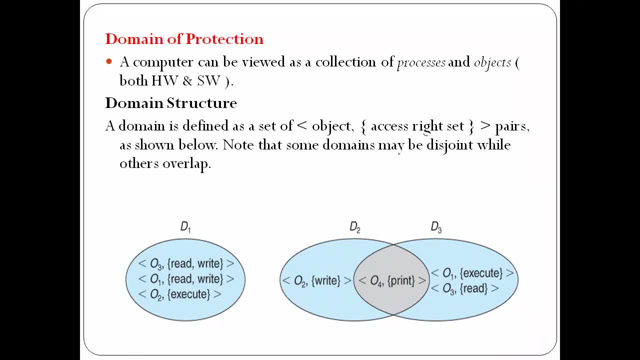 so here, if you take a small computer, it consists of two domains. one is hardware domain, next one is software domain. i already told what is the meaning of domain. domain is nothing but particular category. domain is nothing but collection of categories. so simply, if you take a normal 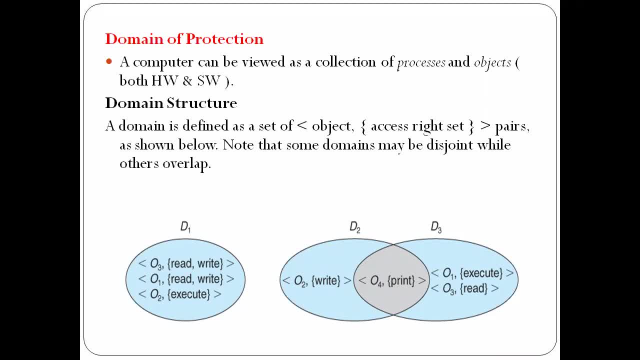 computer, normal computer, consists of two domains. what are those? software domain and hardware domain, for example. if you take, for example: uh, my mouse is paid in my computer, my mouse is paid, okay, now, uh, which domain is tell you in my system? respond anyone, for example, in my system. 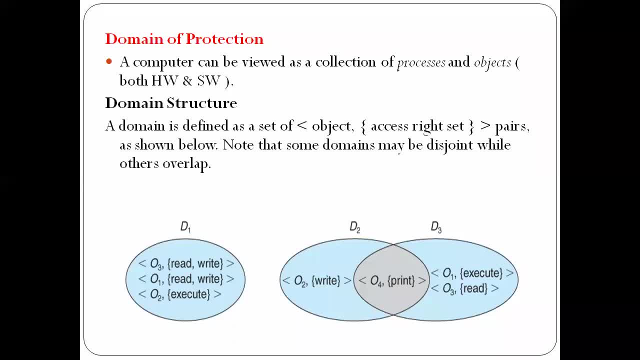 my mouse is paid, my mouse is not operating well. now respond anyone. okay, so which domain is failed in my system? which domain is failed in my system? second, third, fourth, five, six, seven, eight, nine, ten, eleven, twelve, 13, fifteen, 15, 16, 17, 18. 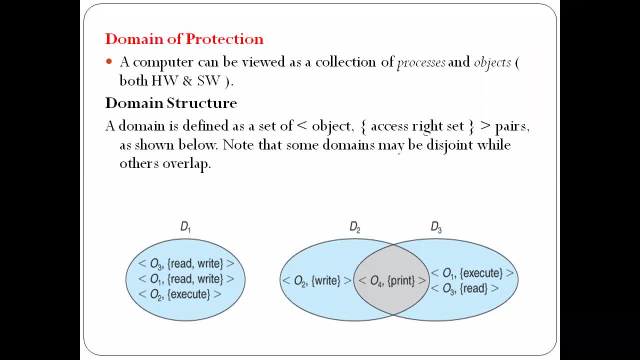 19, 20, 21, 22, 23, 23, 24, 25, 26, 27, 27, 28, 28, 29, 31, 28, 31. next one is software domain. now, if my system mouse is failed, which type of domain is failed? 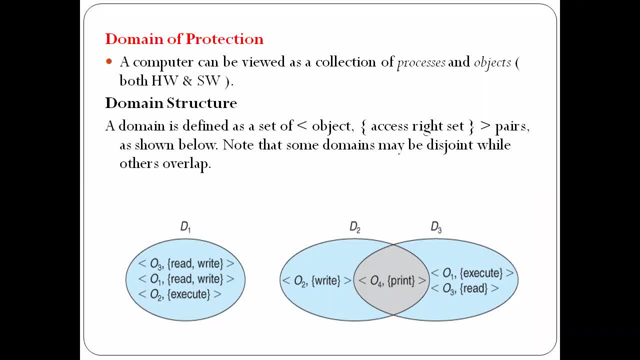 either software or hardware. different a domain failed in it. my system consists of two different types of domains. first one is hardware domain. next one is software domain. software domain is nothing but operating system, something my programs. hardware domains are nothing but all the hardwares in the system, all the hardwares in the system. it 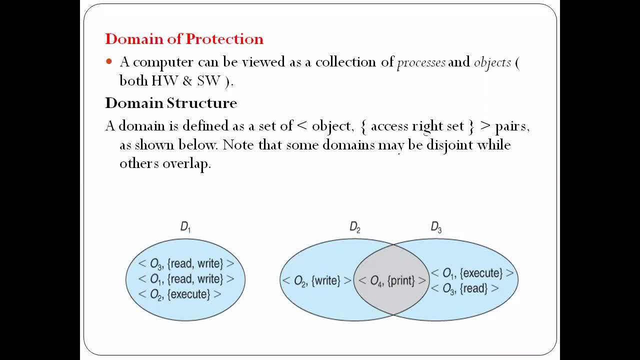 may be a mouse, it may be keyboard, it may be something like this: hardware devices. and now my question is: if my system's mouse is failed now, which type of domain is failed in my system? hardware, sir. hardware, yes. hardware domain is failed. now respond anyone. for example, in my system, ms office is not working properly. which domain is failed? 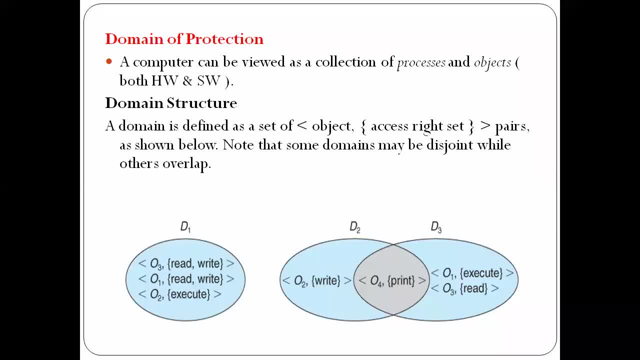 software. software domain is failed. so simply, yes. what is the meaning of domain here? domain is nothing but particular category. each and every computer is viewed as collection of process and objects. here, process is nothing but software, objects are nothing but hardware. so simply we can say: every computer is viewed as two types of domains. first one is hardware domain, next one is software. 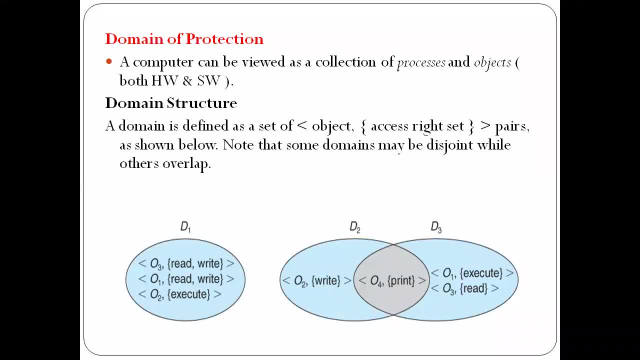 domain. so that is the meaning of domain. now, coming to our domain structure, coming to our domain structure, what is the meaning of how it is domain is organized, how this domain is organized in any system. so what is the meaning of domain here? here, domain is defined as set of objects. 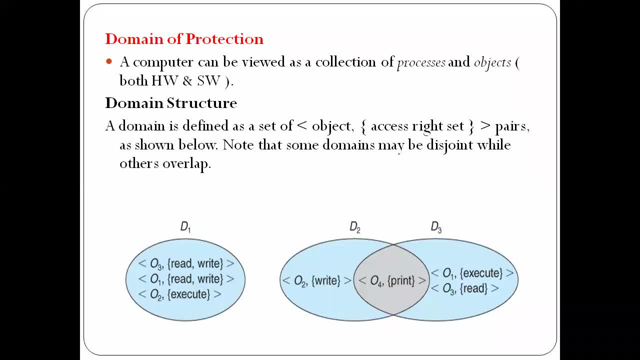 access rights and also page and also page. domain is nothing but the domain is organized. nothing but domain is different as set of objects. okay, access rights and also page. okay, so look at this diagram. there are three domains, are there? there are three domains on there. what is that? this is my objects. d1 is look like as my object. okay, for example, 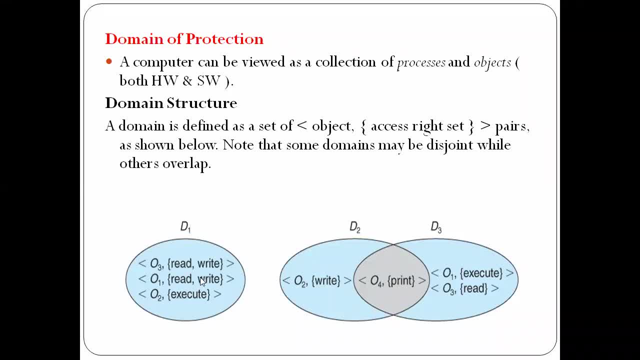 one is object to render demo access permissions to remove demo parent. but yes, what is the meaning of this? okay, what is the meaning of this? so d1 is one domain, d1 consists of three objects and d1 consists of three objects. what are those? so object one consists of read android. object two: 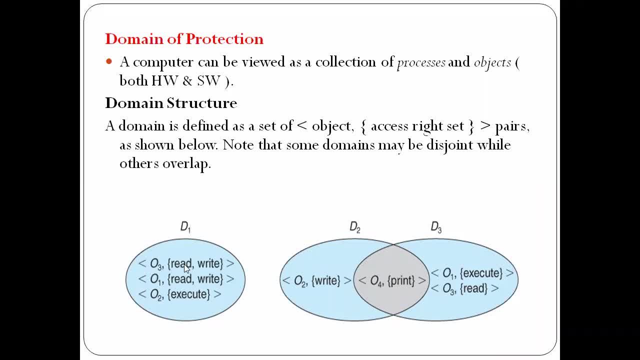 consists of only execute. object three consists of uh- read write now. d2 consists of only object that is auto object. that is right permission. b3 consists of only uh object one, object three, and that is object one is execute. object three is uh, that is read permission now. 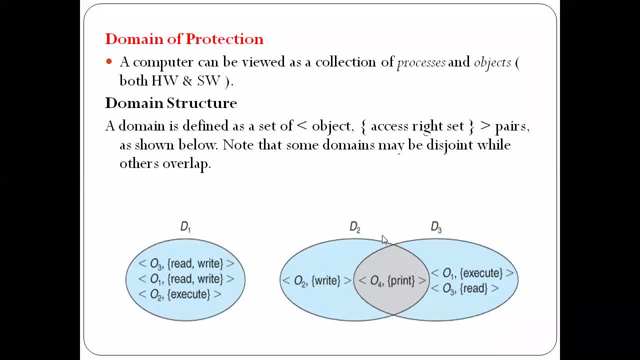 here. this is the pair. what is the meaning of page here? pair is nothing, but here d2 b3s are overlapping each other. some part of some part of d2 b3s are overlapping, that is the overlapping part is nothing. object four: overlapping party is nothing but object four. now here. object four consists of: 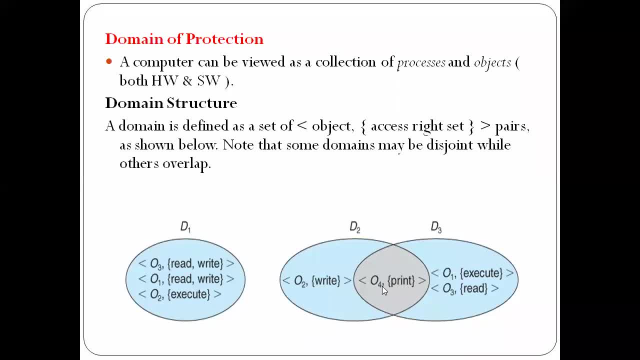 a print permission. what is the menu of information? so this operation can perform domain two under domain three, but not domain one. i mean that. so domain one consists of their own task. their domain two consists of their own task. domain three consists of their own task, but in some cases okay. 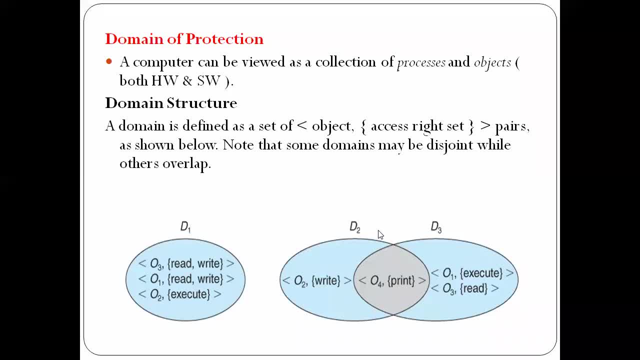 uh, two or more domain consists of the same task that is overlapping. this is called as pay, this is called as paid. so in this small example, domain one consists of their own tasks. domain two consists of their own task. domain three can start their own task, but here domain two. domain three consists of: 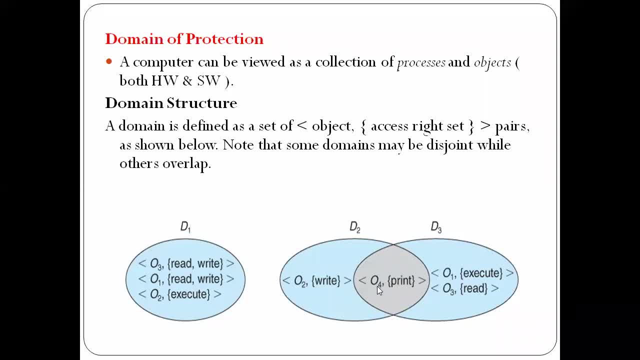 one common one common object that is object for token object, so that is print, that is print, so printing. printing arcs is used by domain three as well as domain two. this is not only- this is not only uh property of d2 and bp, this is the common property of d3 and d4. they can use, okay, this one method, but option four can. 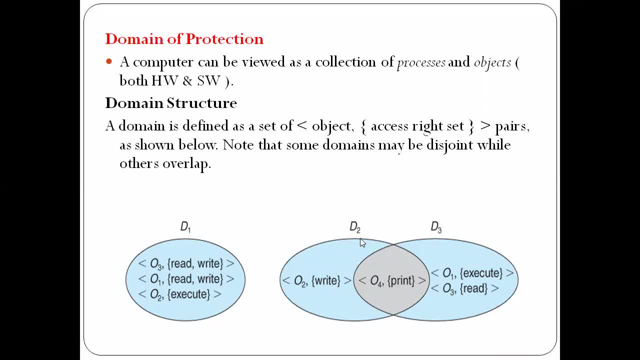 use d3 as well as d2 also. so this is in the meaning of domain structure. so what, what you have observed? so domains are, domains may be individual and also domain may be a shared. so only domains- individual domains- may be individual, like d1. domains may be shared, like d2, d3. so if the object for me d2, d3 series mutual, so even when I'm the 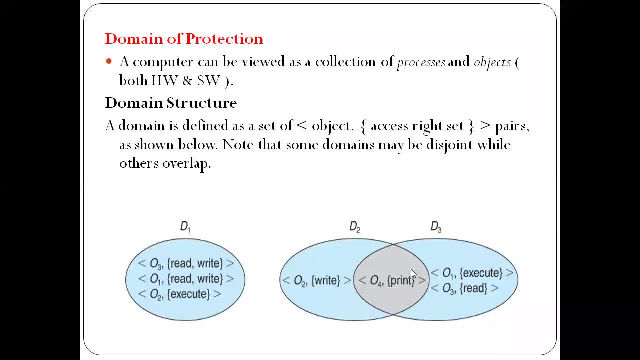 champion. I know this is the meaning of domain structure. simply we can say domains. there are two types of domain structures. there are two types of domain structures. first one is individual domain structure, next one is common domain structure. first one is individual, so here d1 is a individual domain structure, here common. the second one, the common play, the shield, common r. 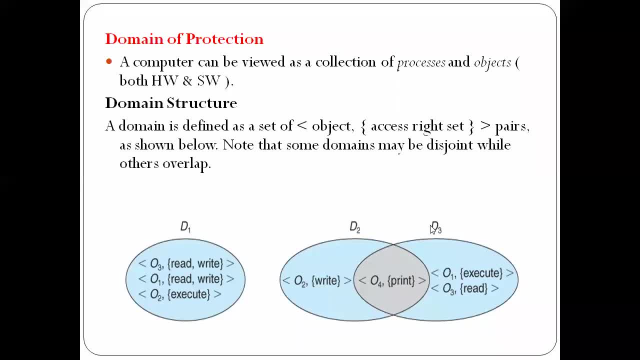 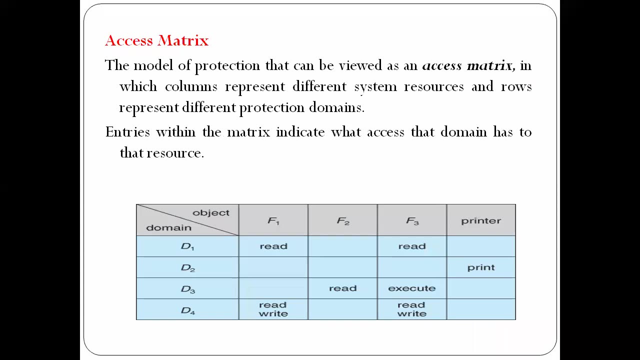 shared domain structure, that is d2, d3, uh sharing, common sharing, common uh object, that is o4, r3. that is the meaning of domain structure. okay, so time is already up. tomorrow's topic, that is axis matrix. okay, we will discuss about this axis matrix by tomorrow. okay, syllabus is completing. okay, in. 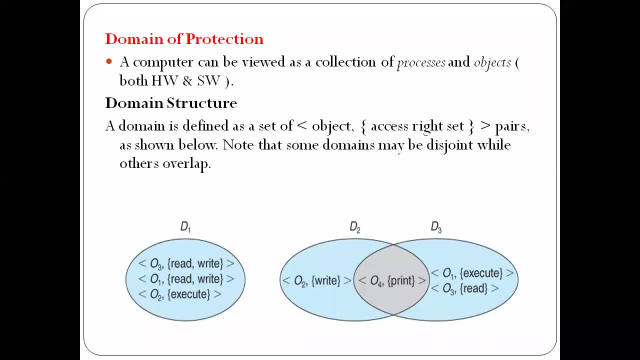 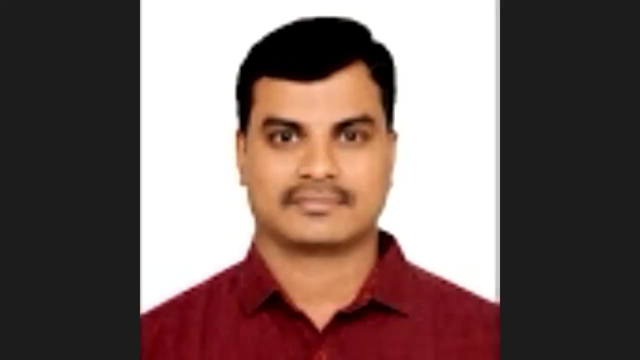 this week we will complete our 58. 15 it is very small utility. 15 is very small unit, so you can give okay. prepare for next class. tomorrow's topic, that is x matrix.